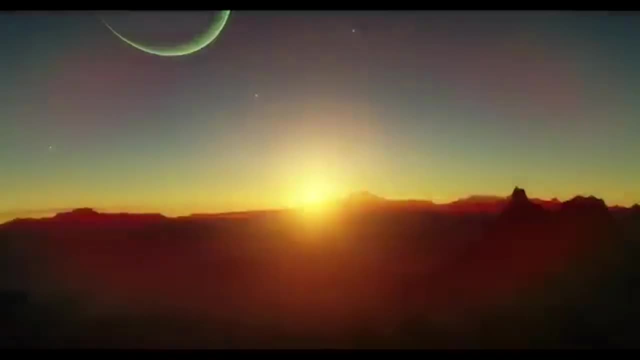 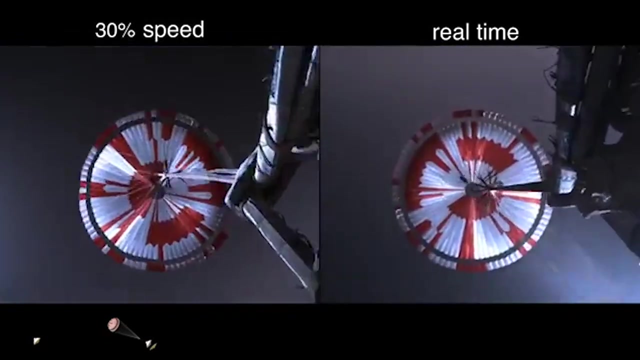 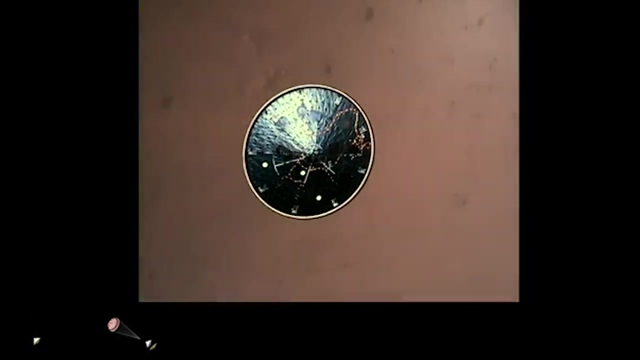 also have secondary atmospheres where gas planets don't. Interplanetary missions to the planets and their moons have enabled scientists to increase their understanding of the solar system more in the past 35 years than in all of previous scientific history. Analysis of data returned from spacecraft has led to the development 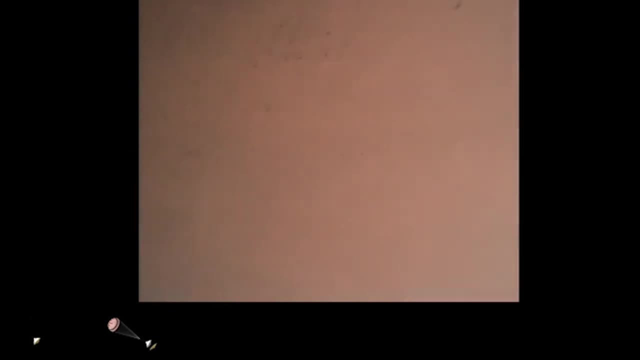 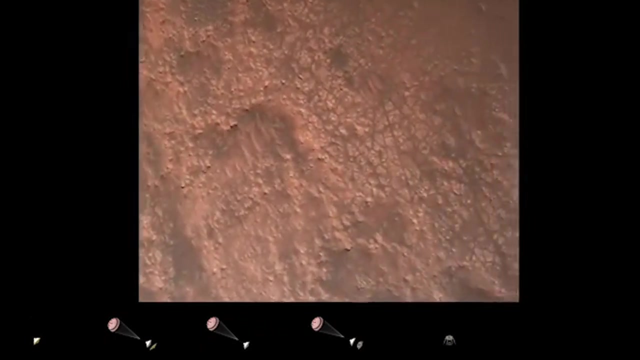 of whole new fields of scientific endeavor, such as planetary geology. We have completed our terrain-related navigation. Current speed is about 30 meters per second. altitude: about 300 meters. We have completed our terrain-related navigation. Current speed is about 30 meters per second. 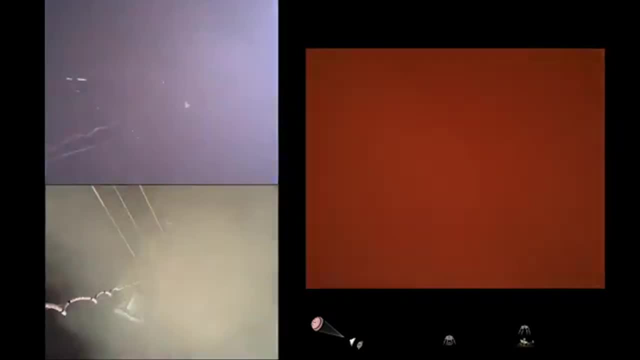 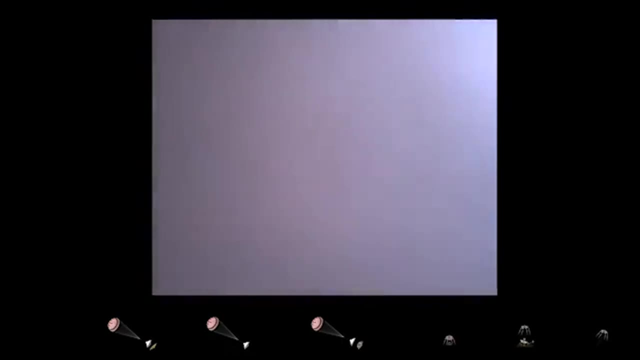 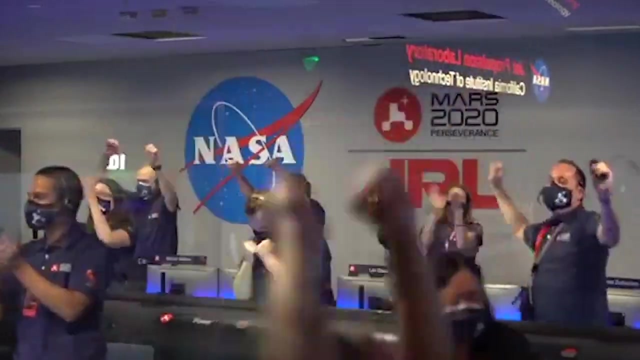 dose temperature about 37 pounds on the surface of Mars. Getting signals from MRO Tango Delta Touchdown confirmed Perseverance safely on the surface of Mars, ready to begin seeking the sands of past life. NASA continues to carry out these planetary missions, including the anticipated return. 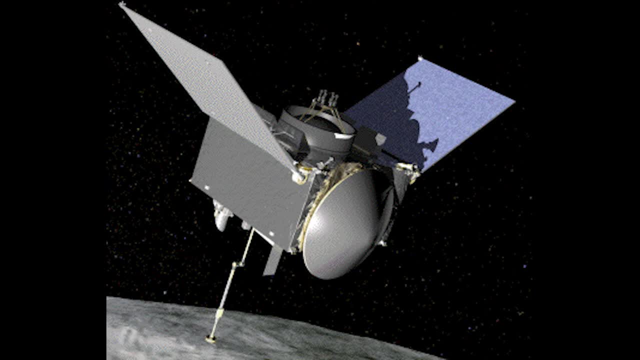 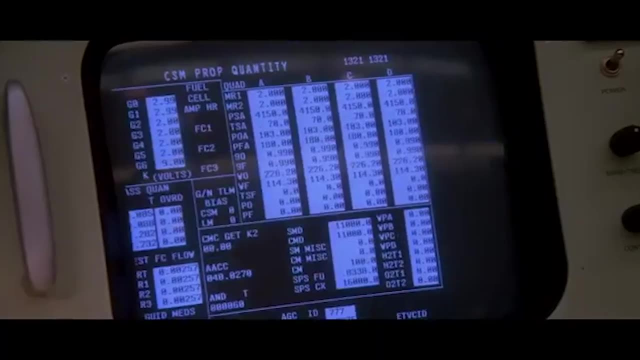 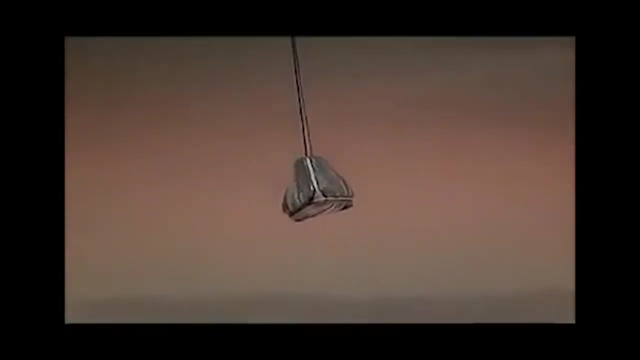 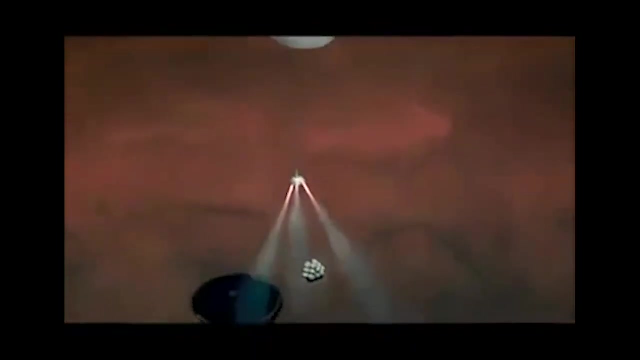 of the OSIRIS-REx spacecraft carrying samples of material from the Near-Earth Asteroid titled Bennu. While there have been a plethora of successes in this 배출 만들committee, some of the To date. a total of 49 missions to Mars have been launched since the 1960s, and almost 35 of them have been failures. 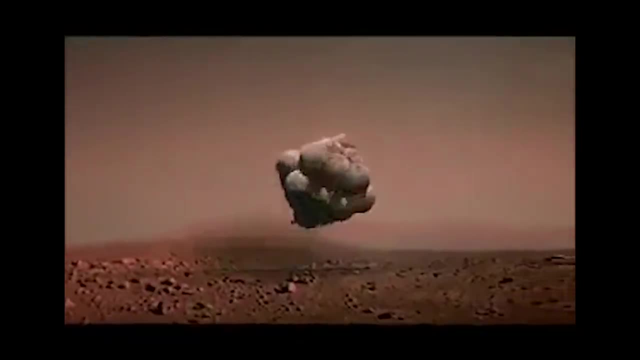 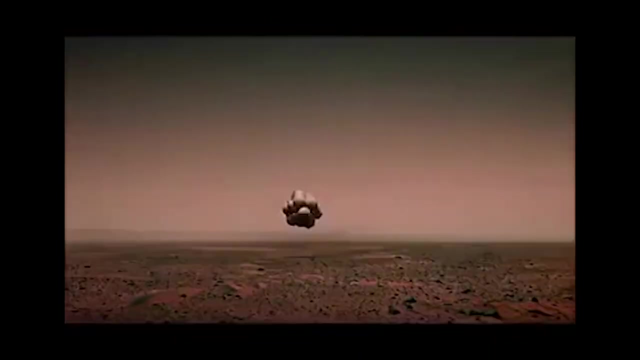 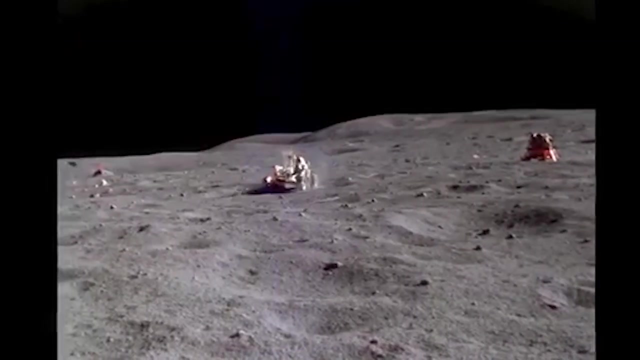 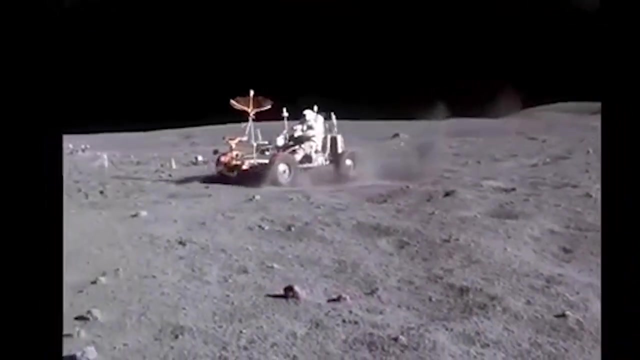 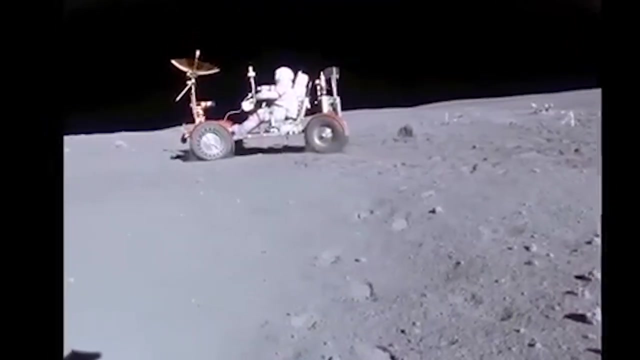 And yet missions to the Red Planet continue to be planned due to the immense scope of knowledge that remains to be gleaned from and about our existence and evolution. The notorious Apollo missions also sought after new discoveries regarding the geological buildup of our Moon. One of the most important missions pertaining to the geology of our Moon was the Apollo 17 mission, where Dr Harrison Schmidt, a professional geology professor and former United States Senator, was part of the three-man crew. 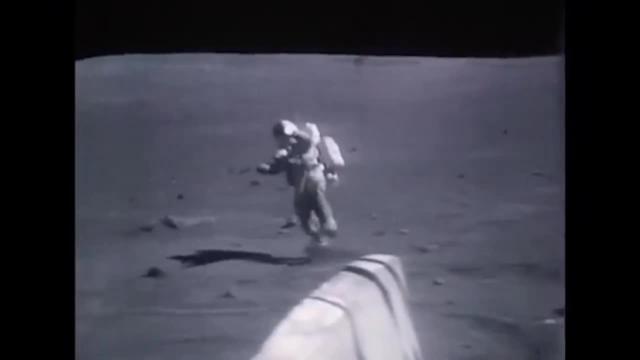 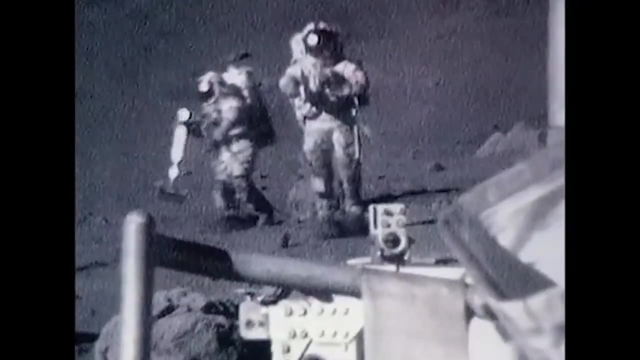 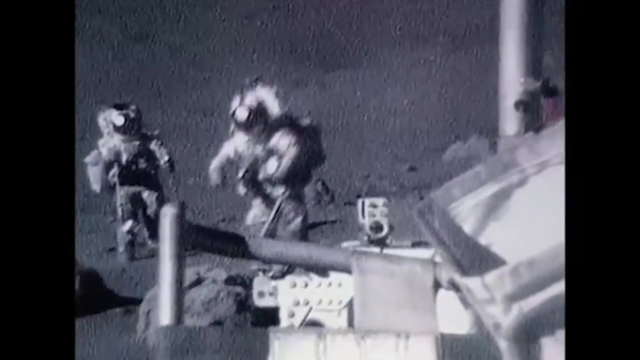 While on the Moon's surface, Schmidt, the only geologist in the astronaut corps, collected the rock sample-designated Tractolite 76535, which has been called, without doubt, the most interesting sample returned from the Moon. Among other distinctions, it is the central piece of evidence suggesting that the Moon once possessed an active magnetic field. 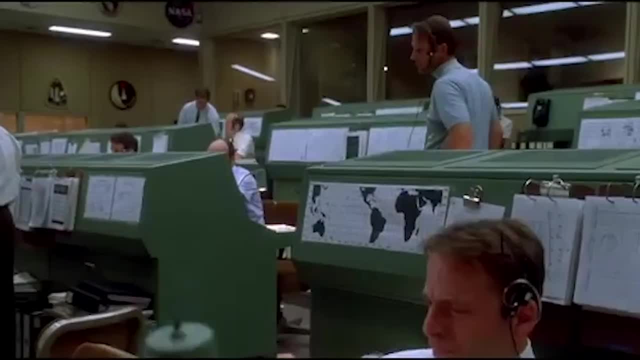 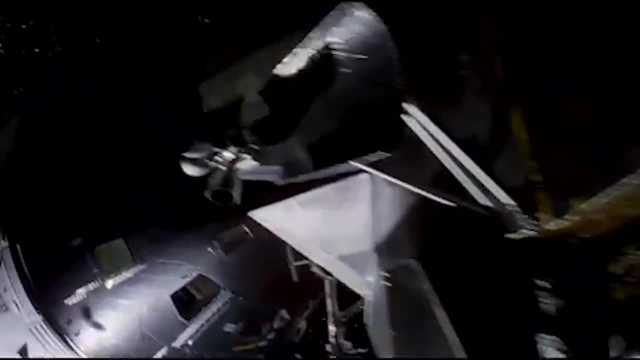 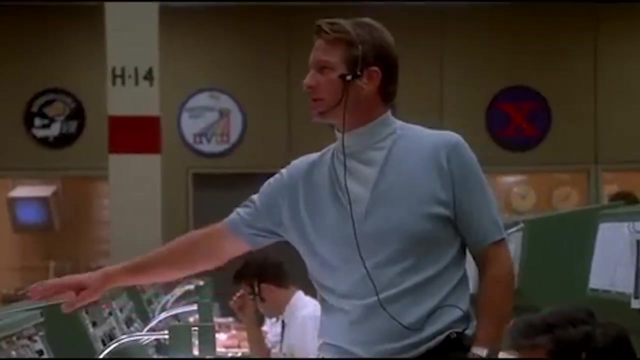 Apollo 13 was to be the third mission to land on the Moon. An explosion in one of the oxygen tanks crippled the spacecraft during flight and the crew were forced to orbit the Moon and return to the Earth without landing. And then, if you could give your oxygen tanks a stir, Roger, that. 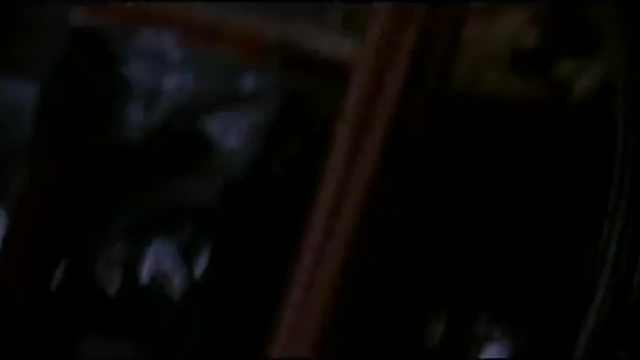 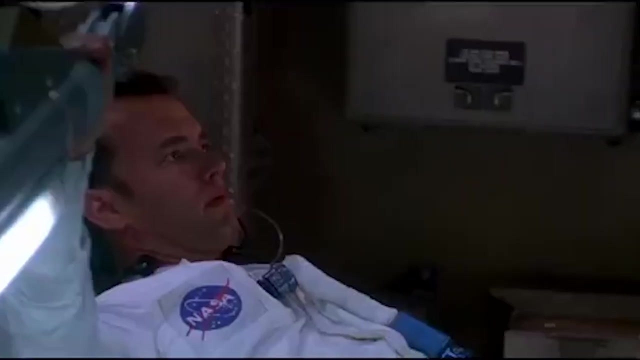 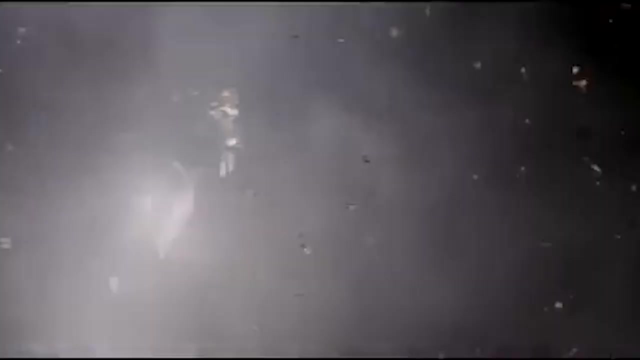 Apollo 13 was to be the second-height mission, meant to demonstrate precision lunar landings and explore specific sites on the Moon. Mission planners were able to focus on more than just landing safely and having astronauts minimally trained in geology gather lunar samples to take home to Earth. 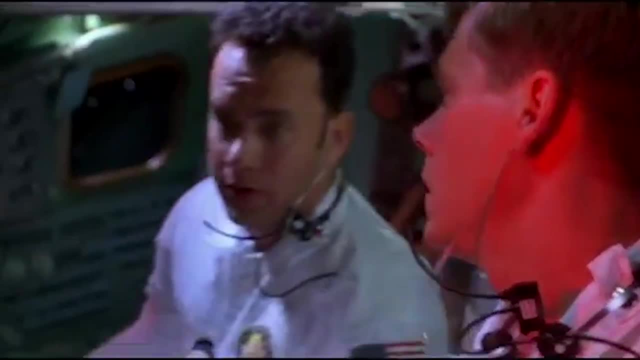 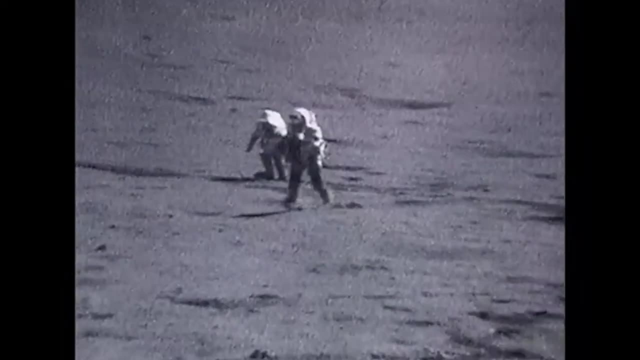 There was a greater role for science on Apollo 13,, especially for geology, something evidence-based. This was emphasized by the mission's motto: While we have made many impeccable discoveries in the field of planetary geology, we still have much to learn. 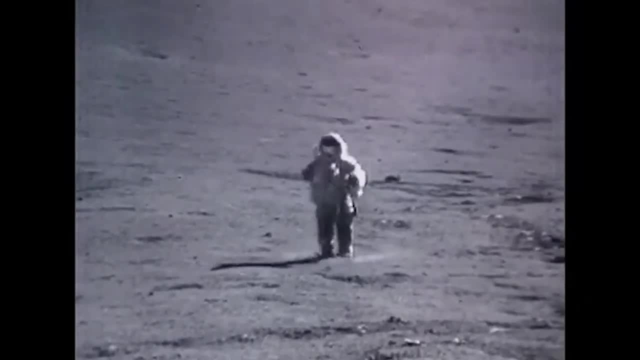 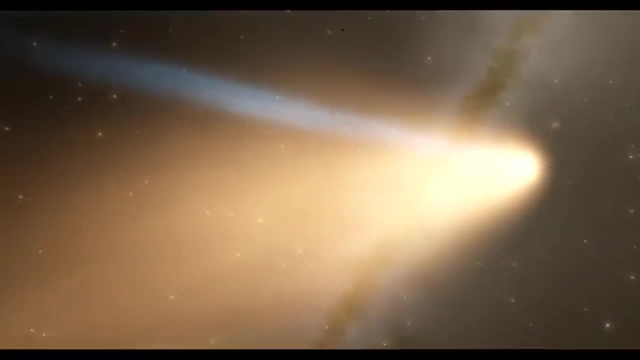 Future manned missions to Mars are thought to be within reach, which will certainly yield amazing results that will change the way we observe terrestrial planets. With great rewards comes great risk, though, and as we have in the past, we will be prepared for outcomes that may not always be successful. 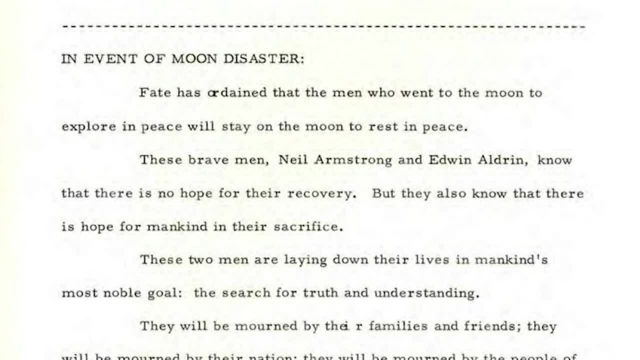 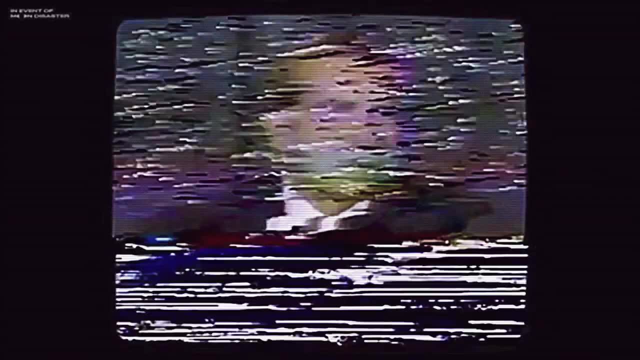 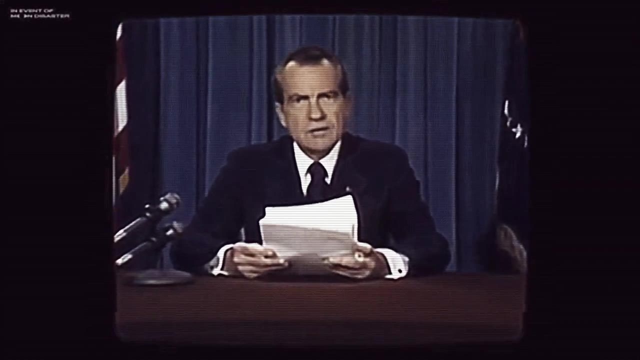 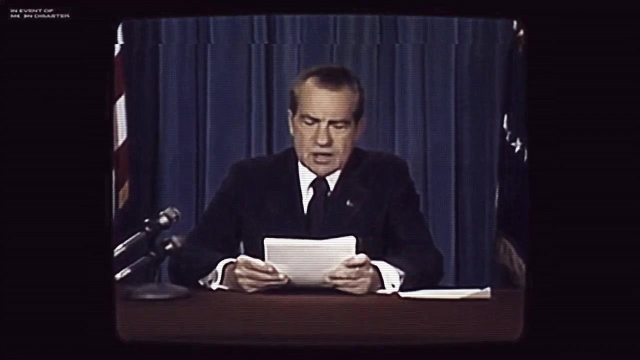 as was President Nixon in his titled speech, in event of Moon disaster. This is the first mission to Mars that has been completed. This is the first mission to Mars that has been completed. Good evening, my fellow Americans. Fate has ordained that the men who went to the Moon to explore in peace will stay on the Moon to rest in peace. 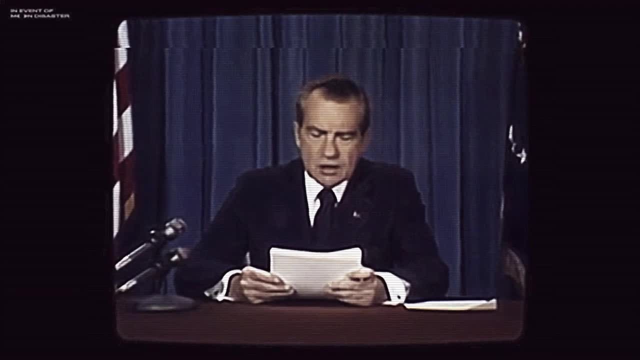 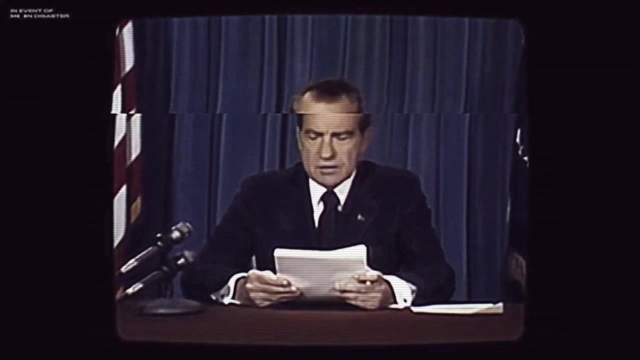 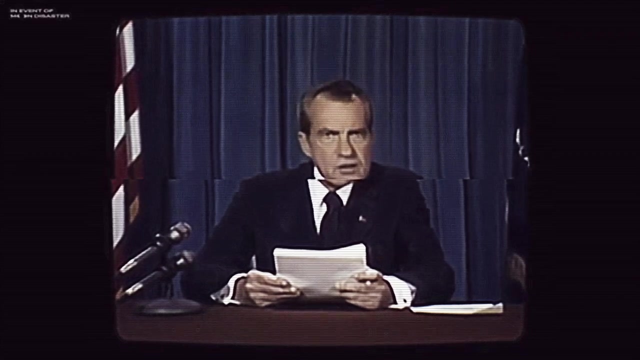 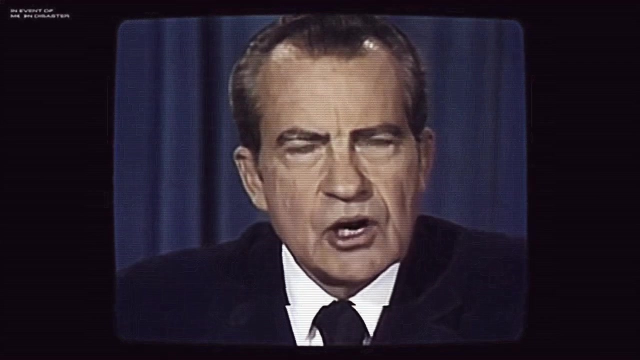 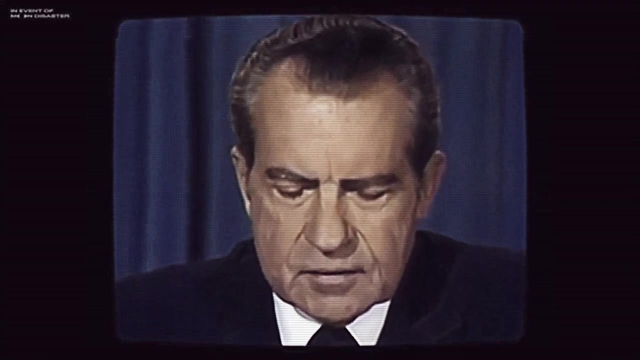 These brave men, Neil Armstrong and Edwin Auburn, know that there is no hope for their recovery, But they also know that there is hope for mankind in their sacrifice, For every human being who looks up at the Moon in the nights to come will know that there is some corner of another world that is forever mankind.